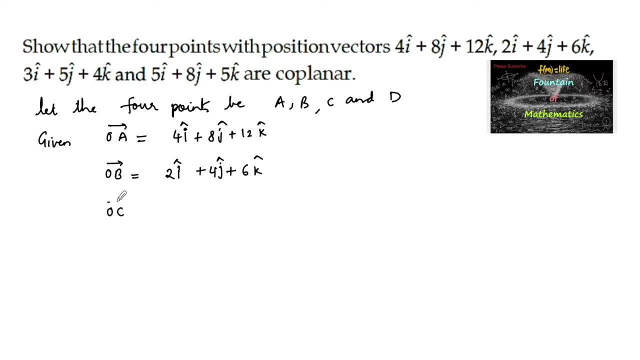 And oc is equal to 3i plus 5j plus 4k, And od is equal to 5i plus 8j. And to prove that these four points are coplanar, So we need to prove that a, b, c, d are points. 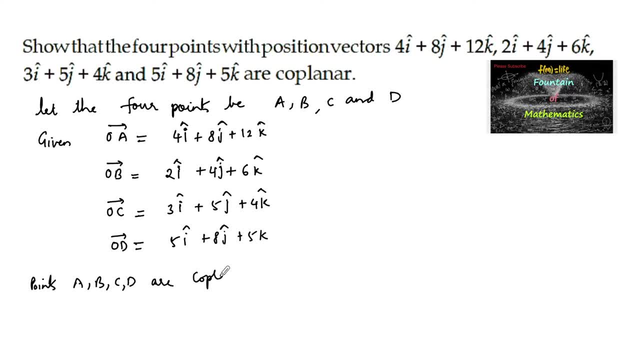 a, b, c, d are coplanar If, and only if, the scalar triple product of a, b, a, c, a, d must be equal to zero. So here we can write: So a, b vector is equal to. 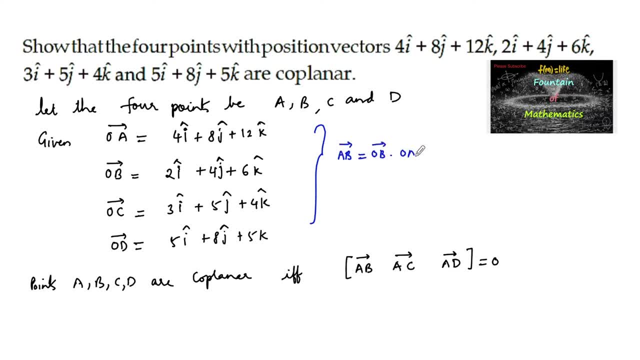 ob minus oa, which is equal to. we can write minus 2i, minus 4j and minus 6k And a c vector. we can write a c vector is equal to 2i plus ab, d, d, d. 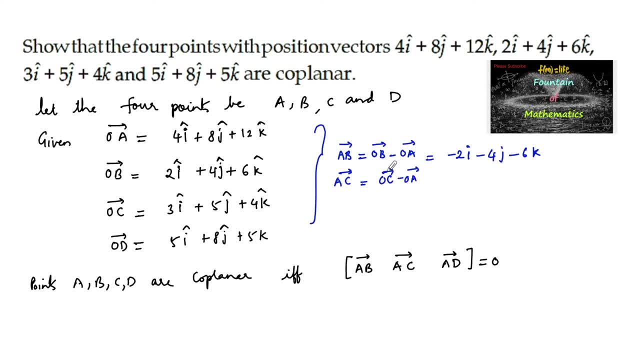 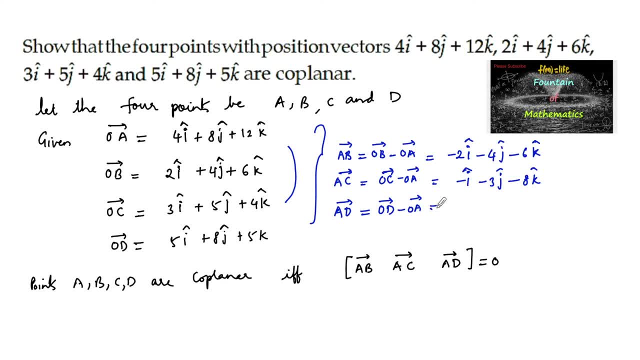 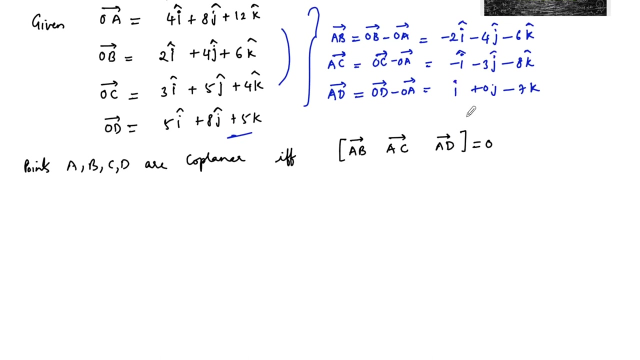 minus OA. so OD vector here and OA vector: 5 minus 4, that is 1 I, 8 minus 8, that is 0 J, and 5 minus 12, that is minus 7 K. so we can write scalar triple product or we can find the determinant of these three vectors: a, B, a C and a D. 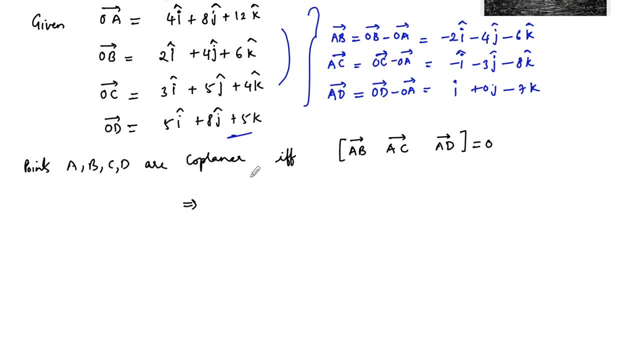 must be equal to 0, so which implies that we can find the determinant of these three vectors, a, B, a C and a D- must be equal to 0, so which implies that- sorry for no leaf- we can write minus 2, minus 4. scalar components of a, B and.